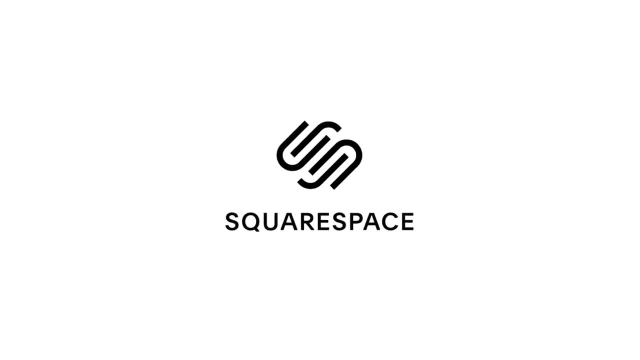 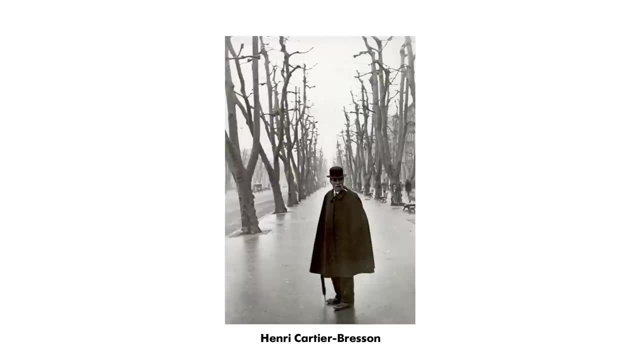 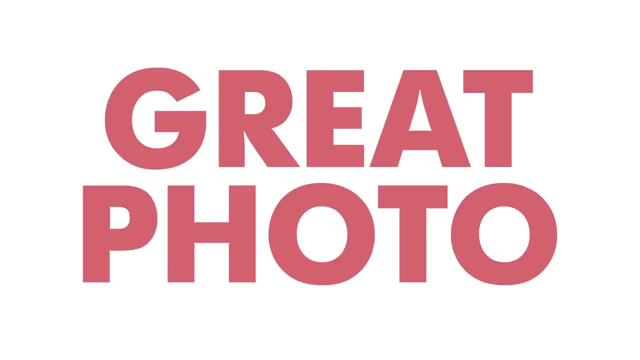 This video is sponsored by Squarespace. If you need a website, a domain or an online store, make it with Squarespace. So you're looking to improve your photography and you're rightfully told that composition is the key to a great photo. You proceed to read up on compositional rules and you realise that 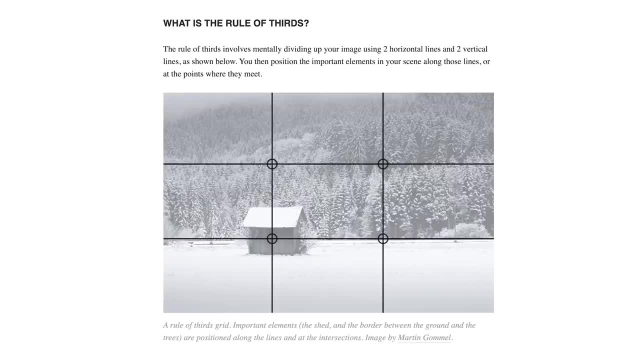 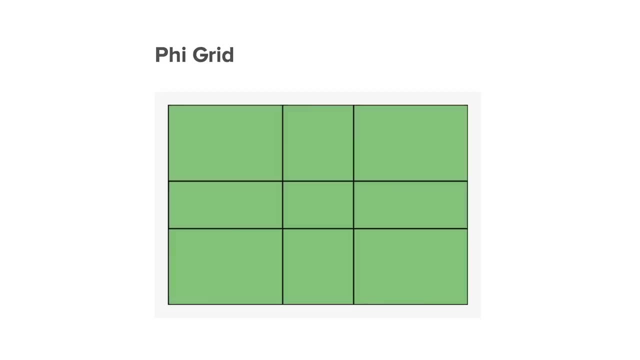 there's a lot to learn. The rule of thirds seems quite simple, but then there's the golden spiral, and you're not entirely sure how to use that. And then there's a grid that looks a bit like the third grid, but it's slightly different, and people call it the five grid. It's got something. 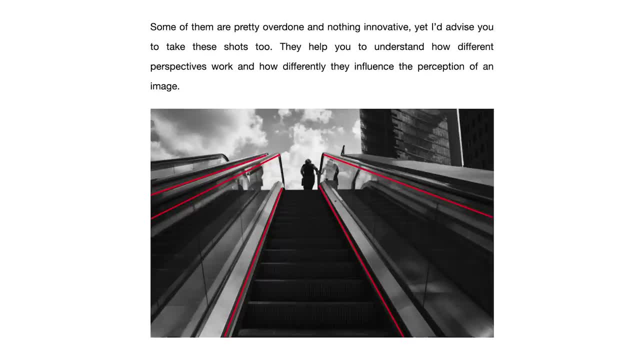 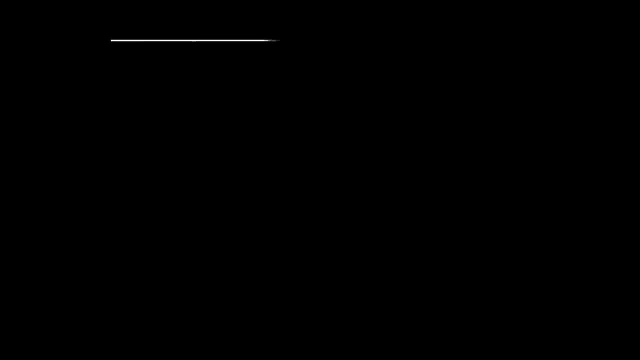 to do with the Fibonacci sequence, but you're not quite sure. Leading lines seem quite simple, but then there are arabesques and leading lines that aren't straight, and then there's dynamic symmetry and you're told about some maths that you don't quite understand and you're not quite. 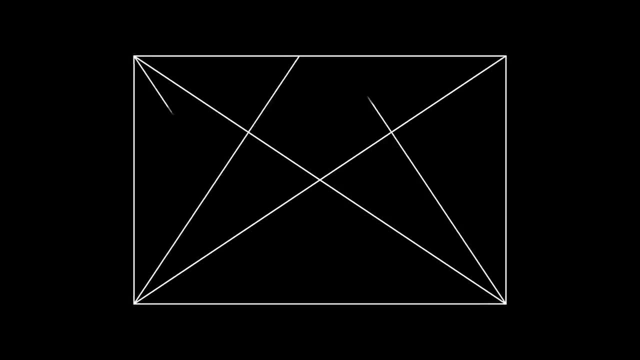 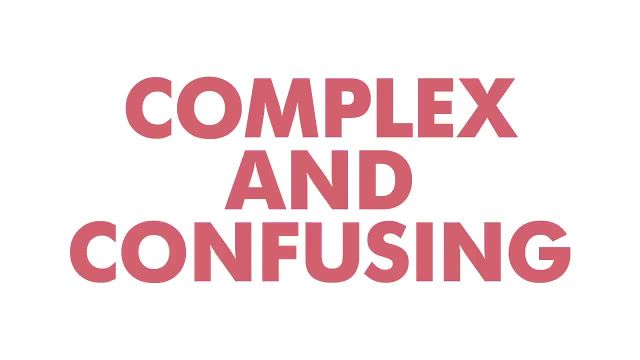 sure how to use the baroque diagonal and the sinister diagonal and the reciprocal lines, And you're shown an Annie Leibovitz picture that seems to be overlaid, with three of these dynamic symmetry grids in a row, and it all looks very complex and confusing. So you decide, maybe. 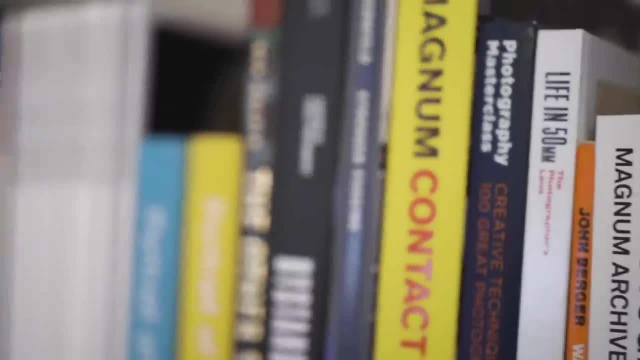 it's best to look at those photos that inspired you to take up photography in the first place and see what you think of them. If you're interested in learning more about photography, subscribe to our YouTube channel and hit the bell so you don't miss a single video. 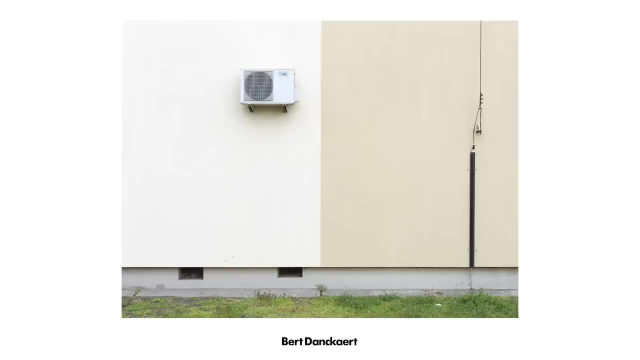 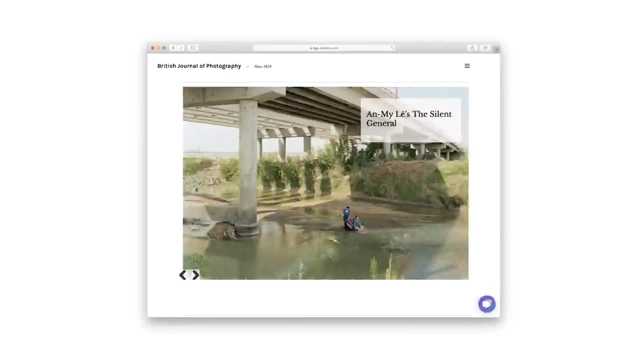 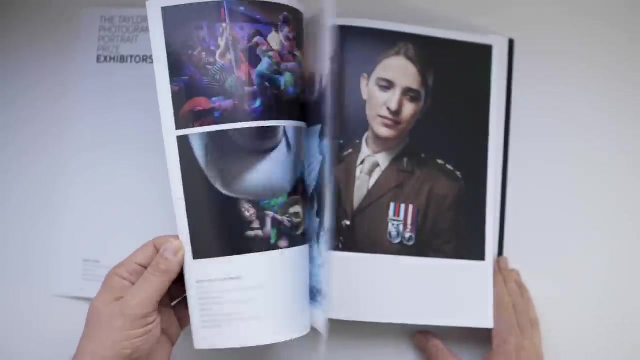 see how these rules apply to them. you examine bodies of work taken by a variety of well respected photographers. you also look at contemporary photographic journals and a wealth of exciting imagery they offer. you look at short lists for prestigious photographic awards, but you rarely find any examples that fit with these rules. in fact, most of these images almost. 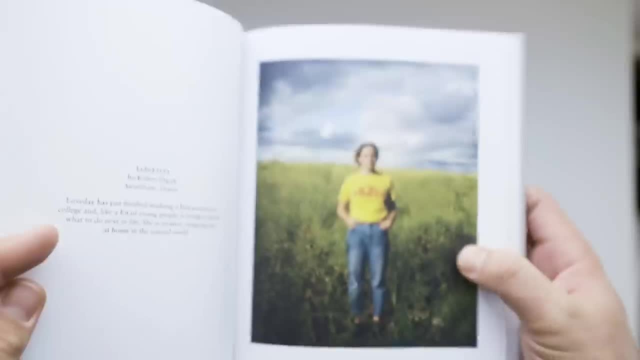 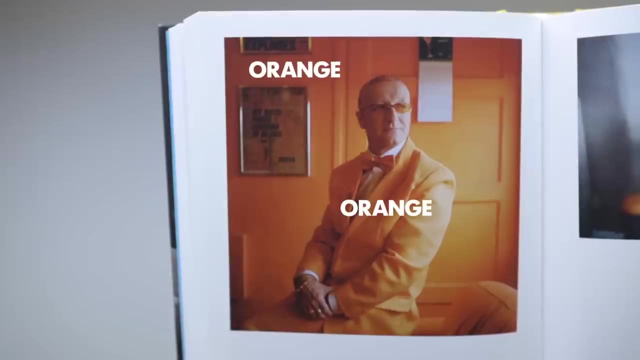 seem to read like a case study of what not to do. weren't you told not to center your subjects? why is there so much empty space above this person? surely this background doesn't help this subject stand out at all by this point. you're confused and you're overwhelmed and you really don't know where to start. 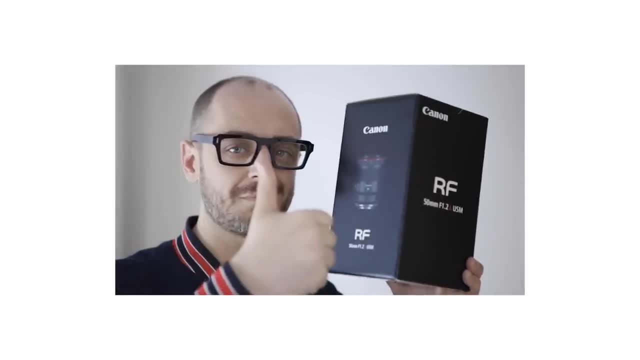 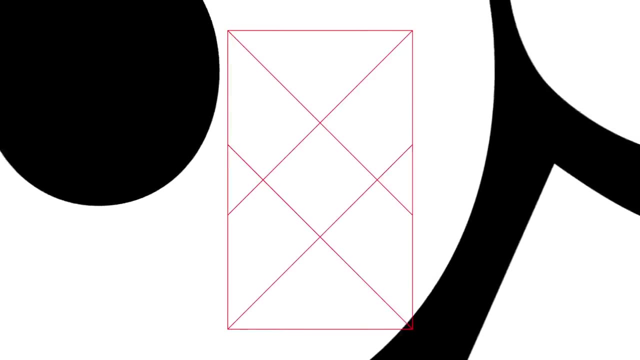 maybe you should just go buy a new lens and see if that helps you take better photos. the problem is that composition is a massive subject and learning all the grid systems and ratios is only one tool in your visual toolbox. i'll probably make other videos focusing on 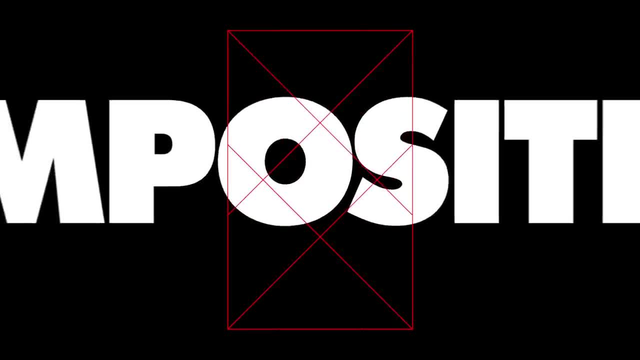 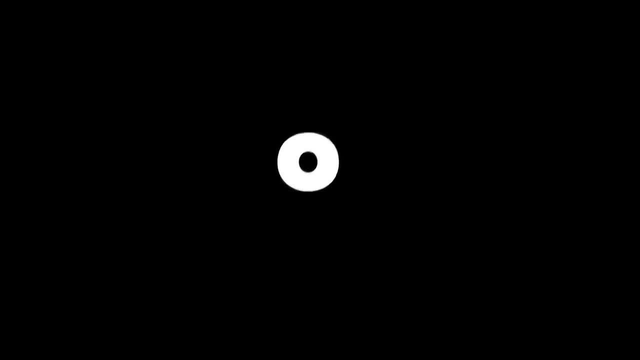 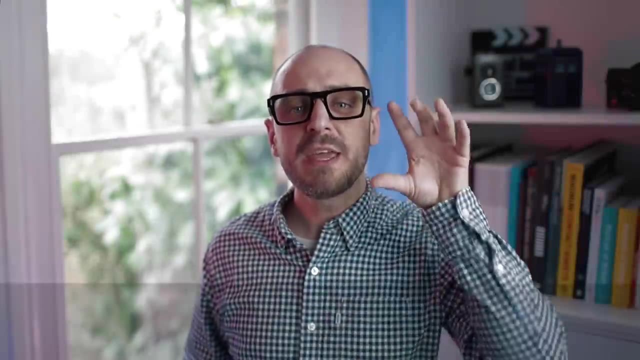 specific elements of composition in the future, but for now, let me give you eight simple tips that will hopefully get you started on improving your composition. number one: get your position right. every representational photograph has two key factors: firstly, the position of your subject or subjects and secondly, the position of the 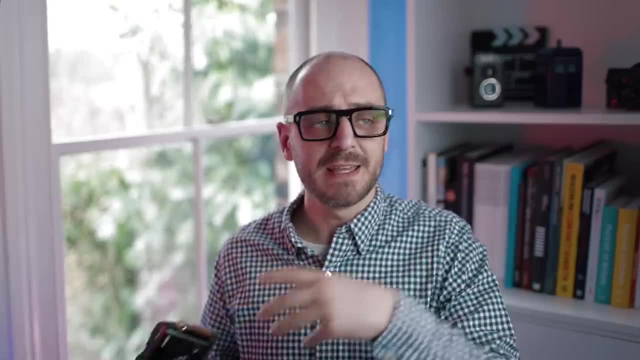 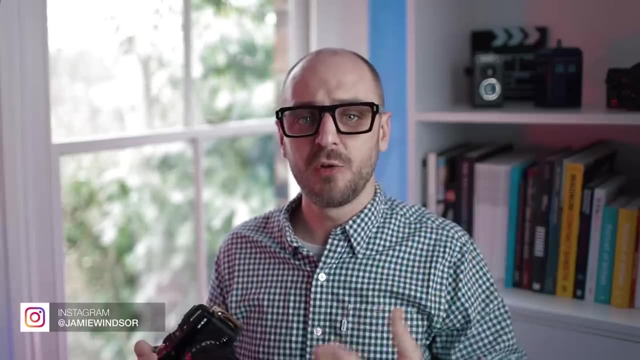 photographer and, by extension, the position of the viewer. now changing either one of these can change how your shot feels, what it means, what story it tells. now, this may sound simple and obvious, but a lot of people really do overlook trying the same shot from different positions. so i'm going to show. 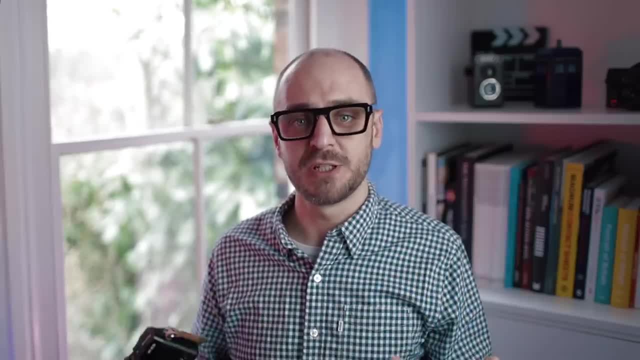 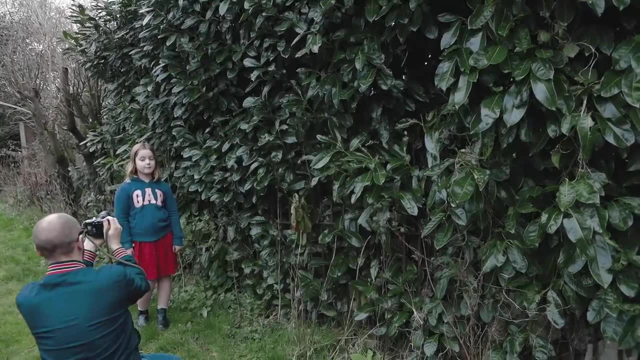 you a couple of examples of how you can change the position of your photograph. don't always default to shooting at eye level. it's how we see the world every day and there's nothing wrong with that, but it's not always the most interesting angle once you've composed your 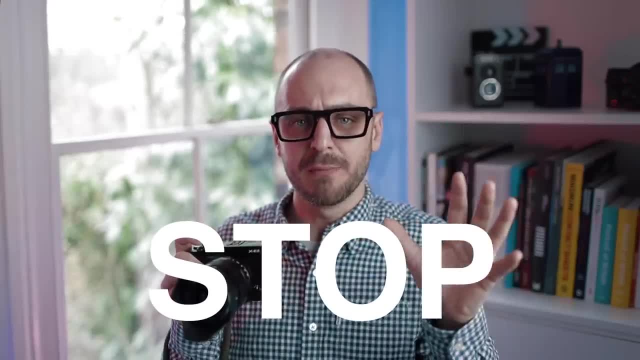 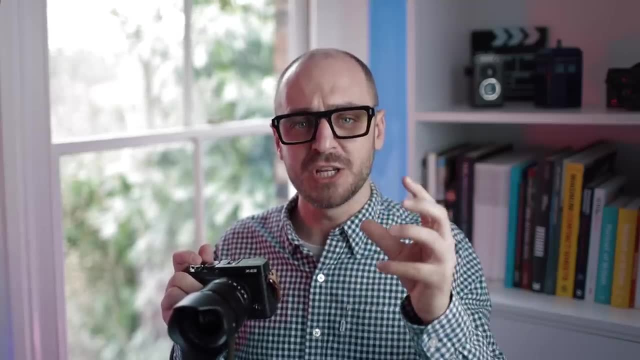 shot. stop. evaluate everything in your frame. is everything exactly where you want it to be? are there any elements or areas that shouldn't be there? if not, change it now. this may mean just taking a side step to the left or to the right. it may mean climbing up something to get. 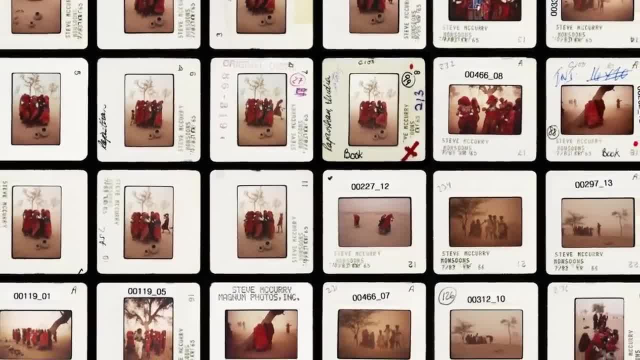 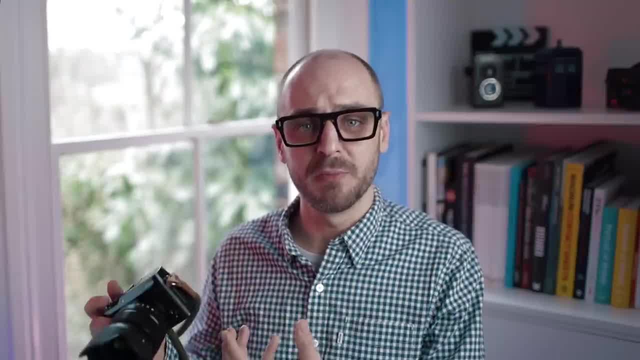 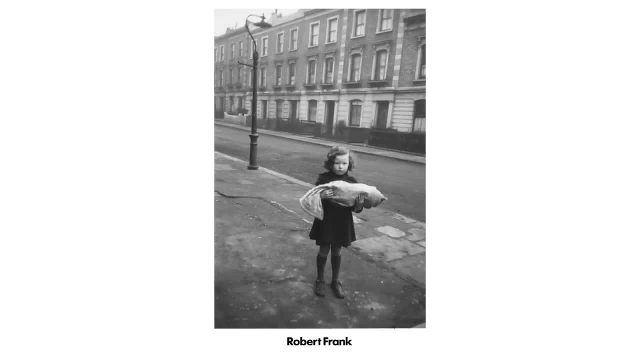 a higher vantage point. it may mean crossing the street. be vigilant and rigorous with yourself. a small bit of effort here can mean the difference between a mediocre shot and an absolute masterpiece. remember to shoot portrait aspect ratio as well. portrait aspect ratio draws attention to objects in the foreground and use landscape format for a more natural feel. 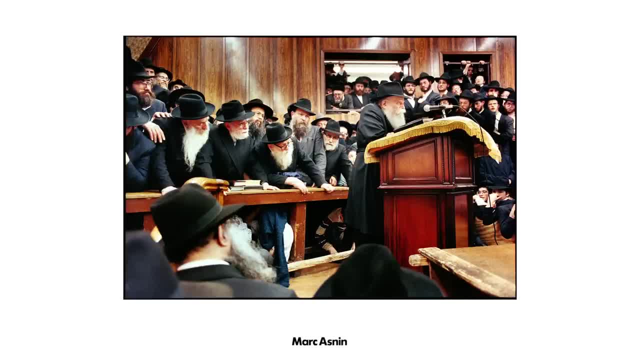 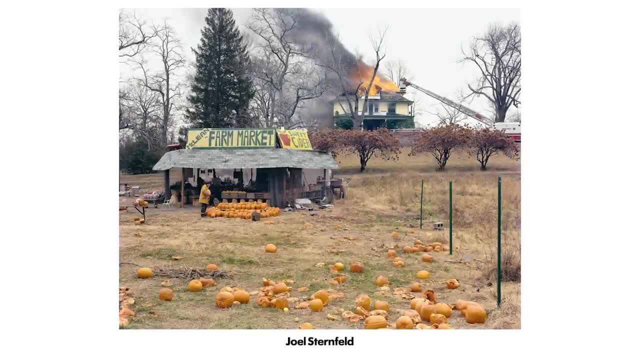 as we often use our eyes this way, unless we're looking up at something tall. take multiple shots in a variety of different ways. push yourself out of your comfort zone a bit. it's all about finding that position where all the elements in your shot work together to create the feeling. 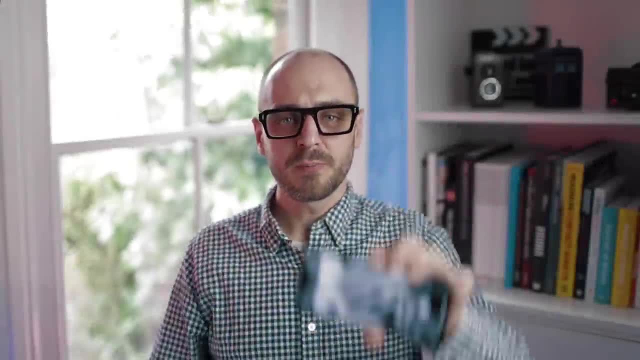 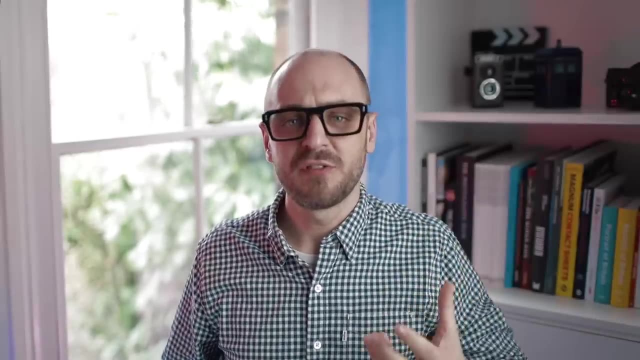 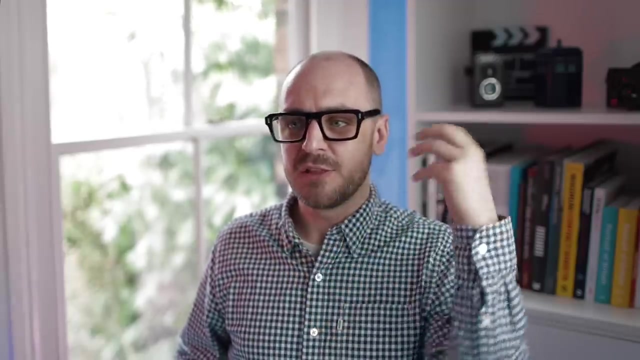 you are aiming for two: use your phone. most of us have a camera phone these days, and one of the biggest hurdles you have to overcome when learning how to compose and visualize an image is being able to translate what we see moving in 3d without these borders, into a still flat two-dimensional 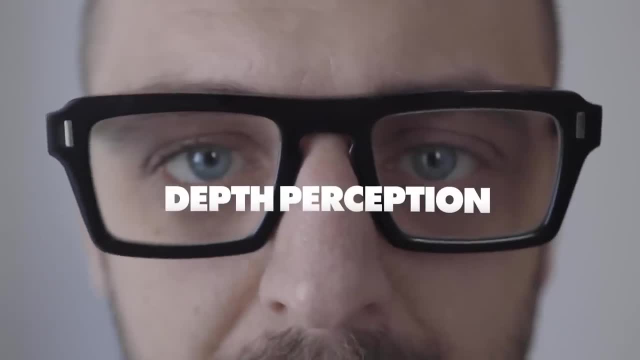 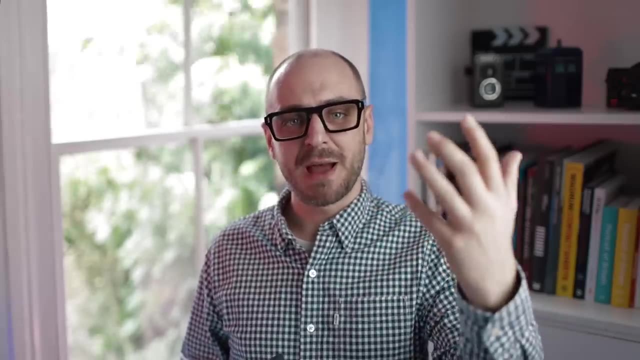 image. because we have two eyes, we see three-dimensionally and so we have a greater perception of depth than a photograph can communicate. our brains can easily filter out distracting background elements because we can see them as further away. but when you flatten that down to a 2d image, those distracting background elements 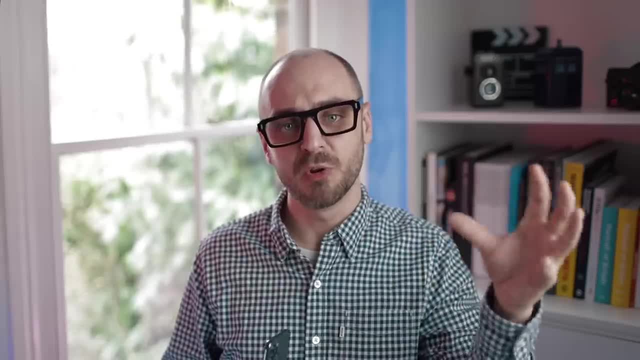 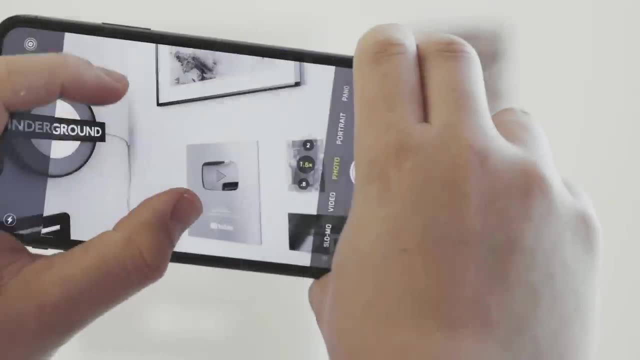 can become much more prominent and take away from what you want the viewer to look at in your photograph. using your phone screen to compose an image can be really helpful. when shooting on my pentax 67, for example, if i'm using a black and white film, i'll often set my phone to black and 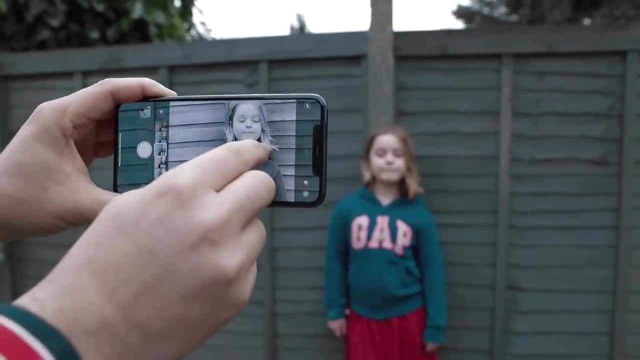 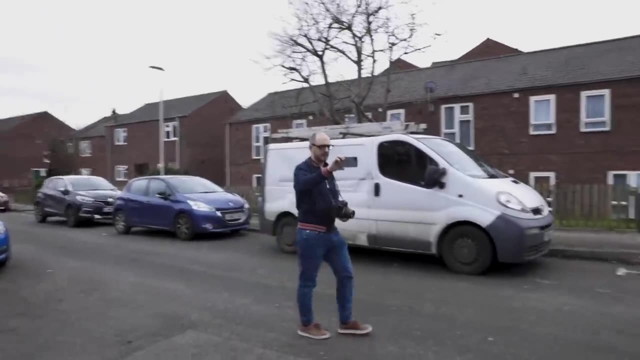 white and i'll pinch into the screen to match the field of view that my 105 millimeter lens offers, which is around about a 50 mil equivalent on a full frame camera. this way i can see the world framed and in 2d i can see how colors translate into tone and i can also tap different. 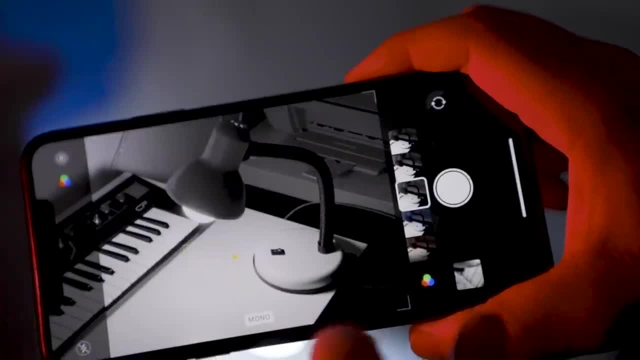 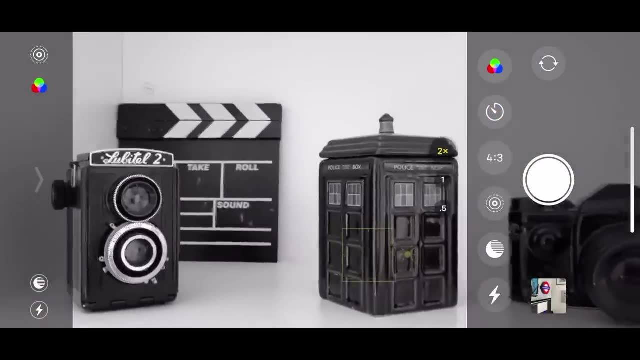 areas of the screen to see how the image would look if exposed for the highlights, for the shadows. this isn't cheating. it's using tools at our disposal to help us get the best shot possible. think of this more like an exercise in learning, the more we practice shooting like this. 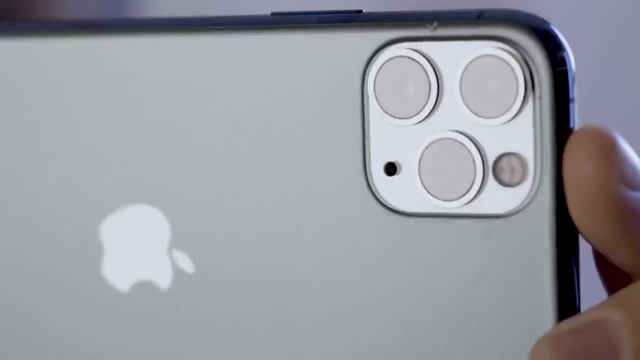 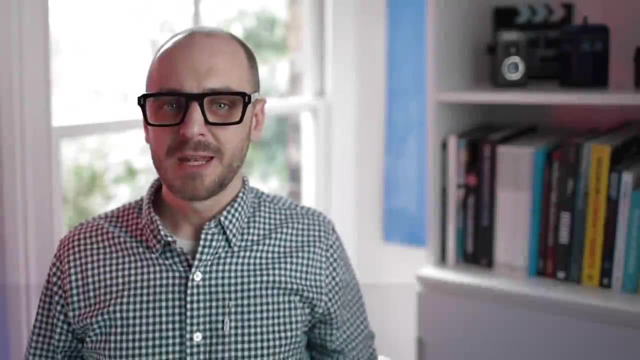 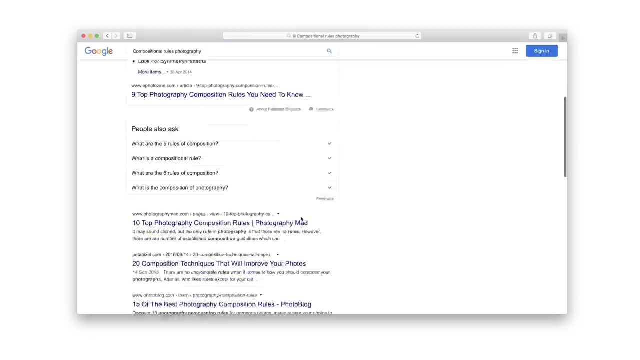 the more we'll start to naturally translate what we see into a 2d composition. it's a great learning tool if you want to improve your ability to naturally visualize a photo in your mind's eye. number three- beware the rule of thirds if you look up any tutorials, articles, tips on photographic. 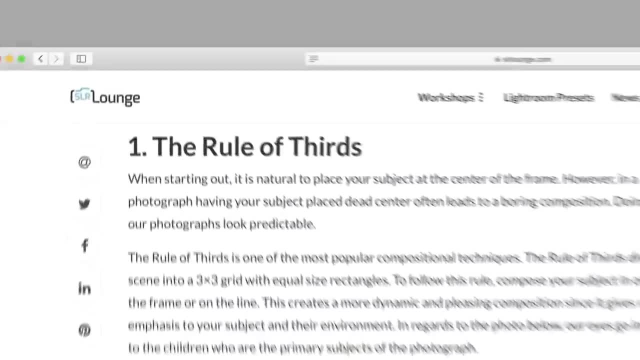 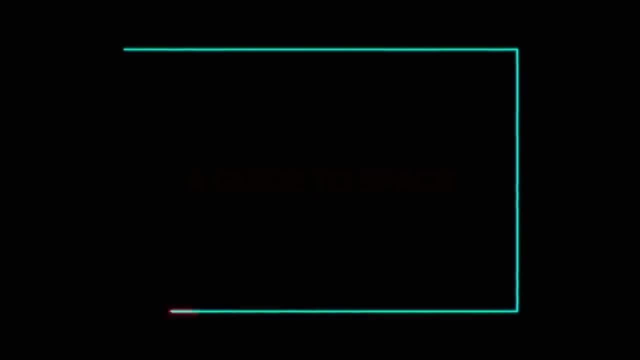 composition, you will likely be met with the rule of thirds right at the top of the list. now, the rule of thirds is a great little shorthand to start you thinking about composition, but understand, just because you place a subject to one of those intersecting points of the grid. 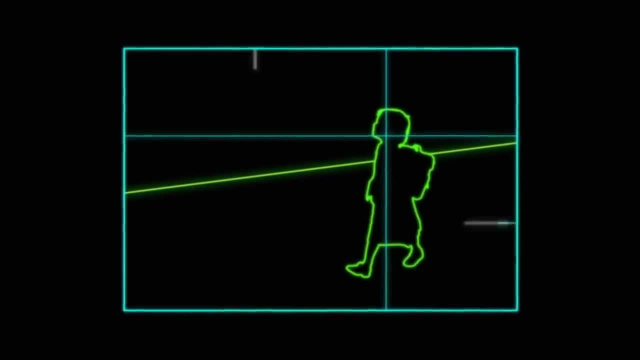 this won't guarantee you a balanced composition. you must think about your shot as a whole. one thing i see a lot when the rule of thirds is used is too much empty space on one side of the image. it can lead to the image feeling unbalanced and there's also more to. 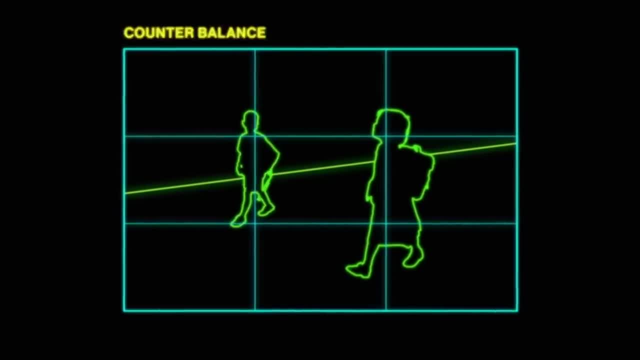 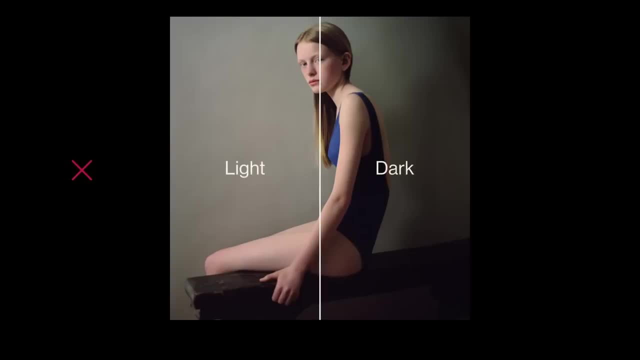 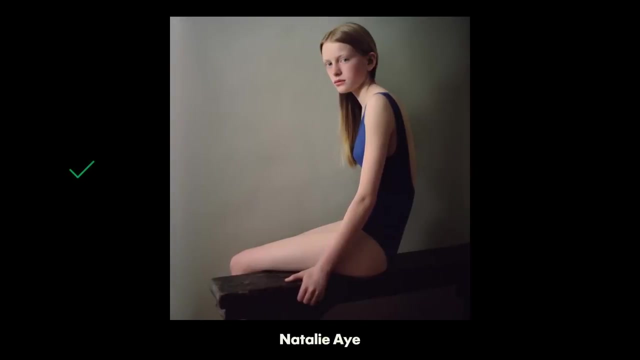 balancing your shot than where you place elements within the frame. tone, color and contrast also all have weight. darkness feels heavier than light. saturated color feels heavier than pale hues- areas of extreme contrast draw the eye. when composing a shot, as well as lining things up mathematically, look for where the areas of contrast are. look. 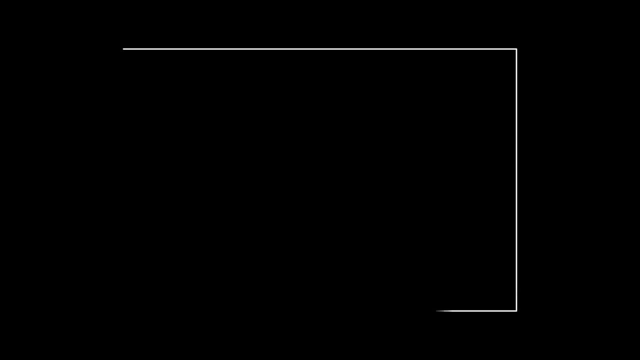 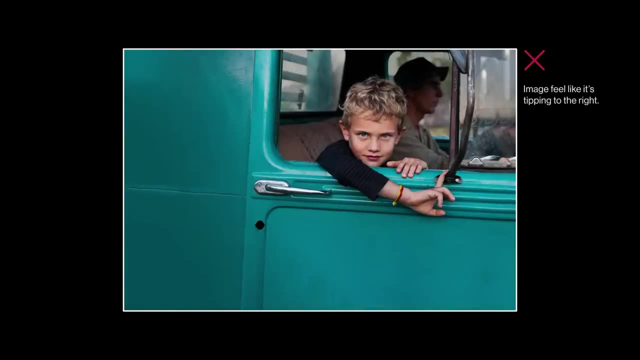 for where the darker tones are. Consider how your image feels as a whole. Does it feel like it's tipping too much to the left or to the right? Consider compositional rules when finding the perfect place to take your shot from, but don't go against your gut feeling If something feels. 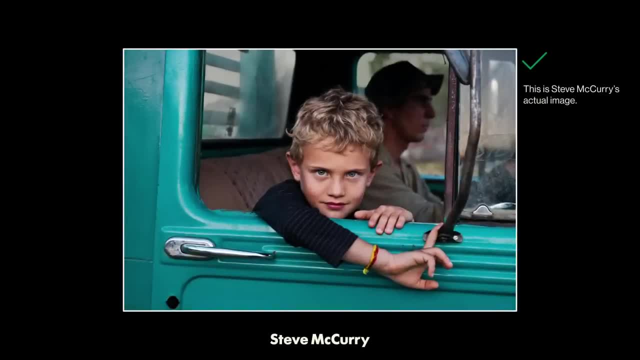 right in a certain place but doesn't immediately make sense to you, then just go for it. There's probably a reason it works that you're not yet aware of. Compositional rules are like a scientific formula. You can use them in art, but first you must know why. If you want your image to look. 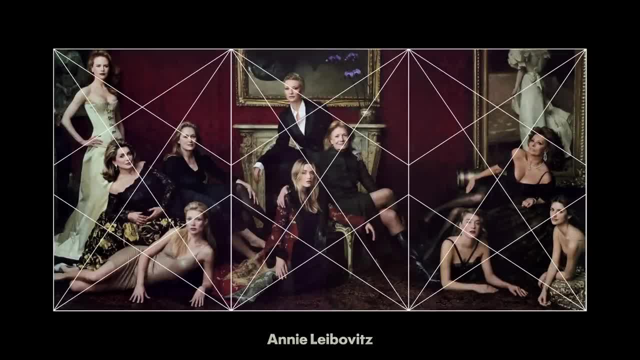 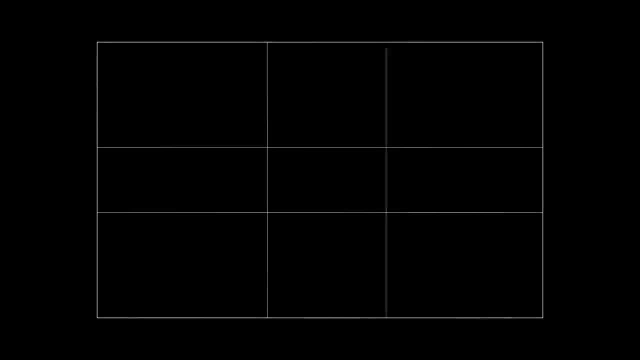 classical use, a classical compositional technique like dynamic symmetry. but you don't need to use these all the time. Learn them, but be mindful about when you use them. Don't fall back on them just because you know them. Think firstly about what you are saying before you decide how to say. 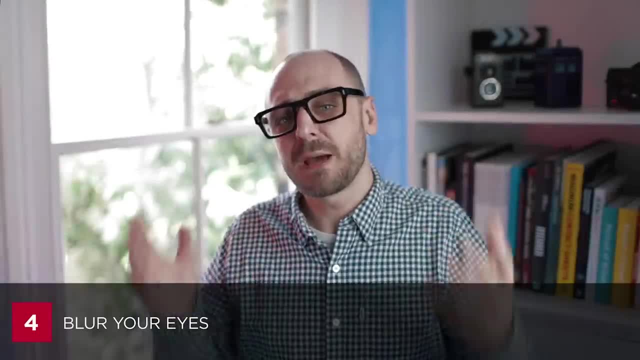 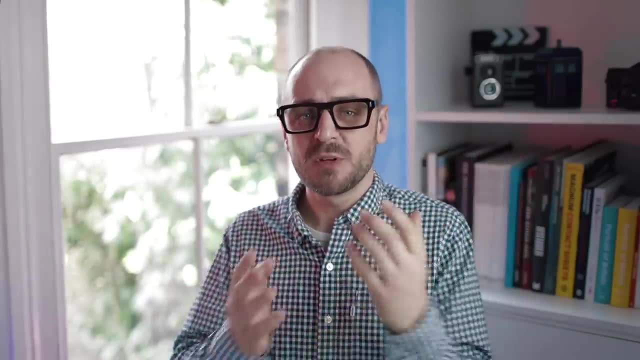 it. Number four, a nice simple one: Whenever you're setting up a shot, squint or blur your eyes. This will help you see abstract colour and shape and form. We're so used, as human beings, to reading the world around us that 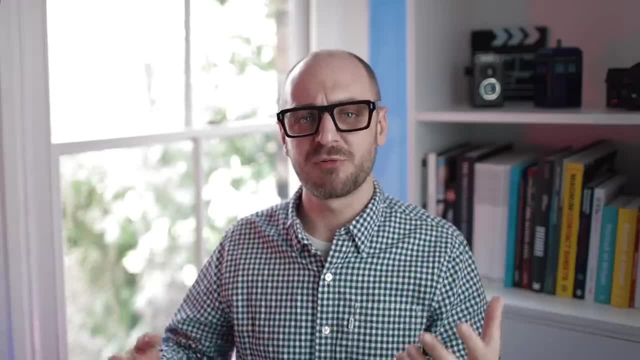 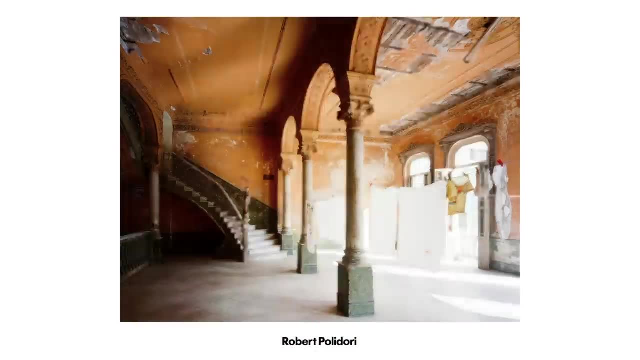 sometimes it's very difficult to take that step backwards and look at it in a more abstract way, but squinting or blurring your eyes will help you see where the contrasty areas are. They'll help you see where the more saturated and the light areas are, and this can really help guide. 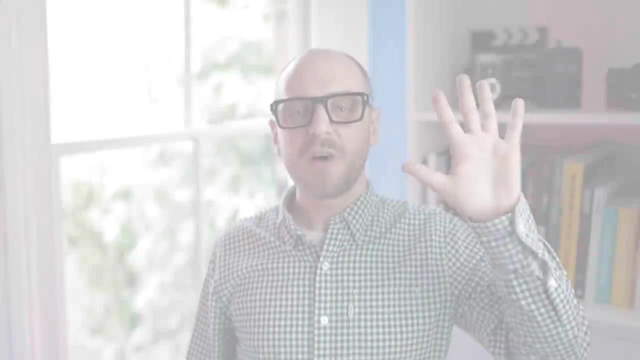 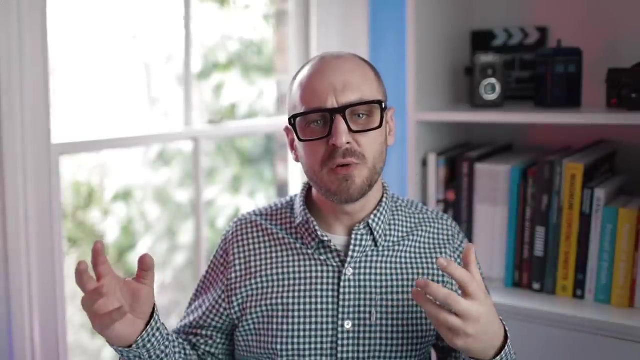 you in setting up a nicely balanced shot. Five: think conceptually as well as aesthetically. Why are you shooting what you're shooting? What do you want your viewers to think about? Think conceptually as well as aesthetically. Why are you shooting what you're shooting? What do you want your viewers to think? 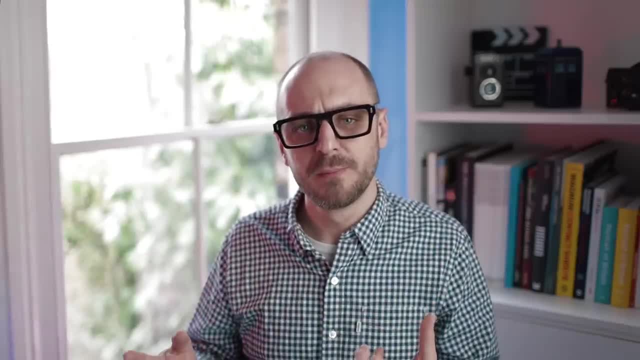 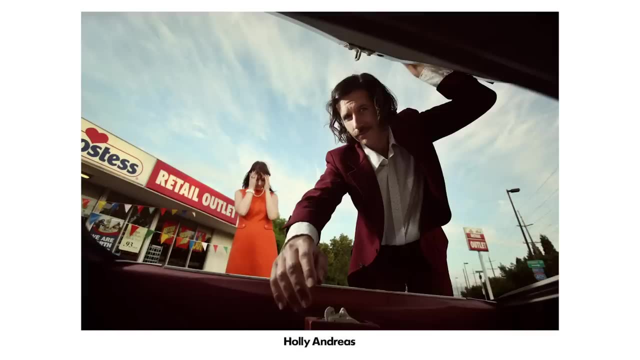 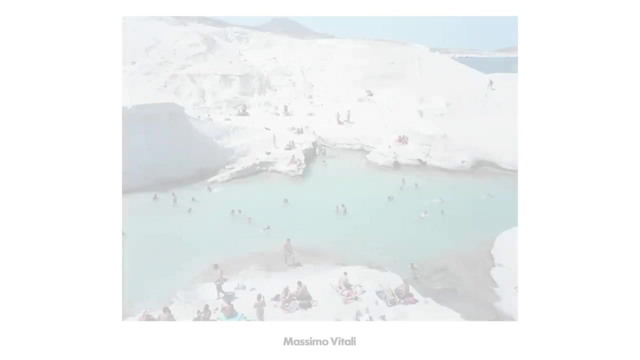 when they see your shot. What do you want your audience to feel? Everything about the way you compose an image will tell part of a story. For example, the angle you shoot from can change how a subject is represented. Being up high, looking down, can detach the viewer emotionally. It becomes more of an overview shot. 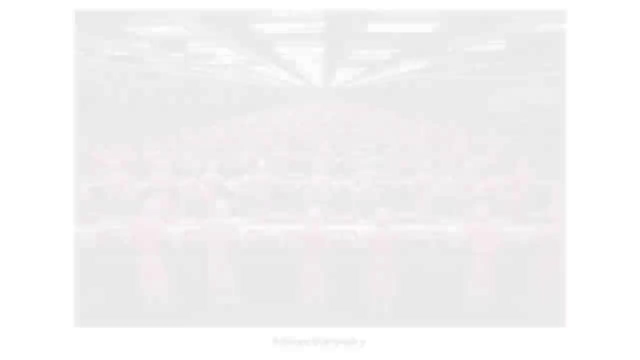 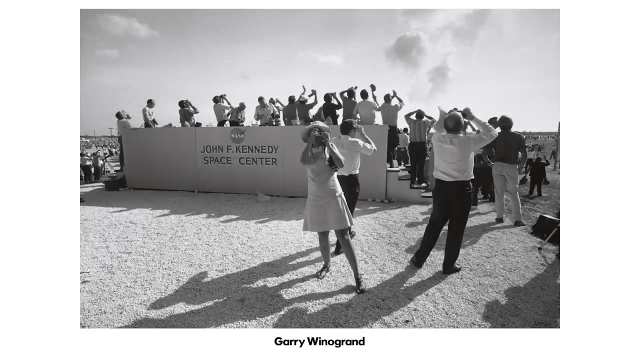 very matter of fact, It's a slightly god-like position, looking down on the world below. The viewer is a privileged observer and not part of the scene. But if you shoot from ground level, then you are part of the scene and by extension. 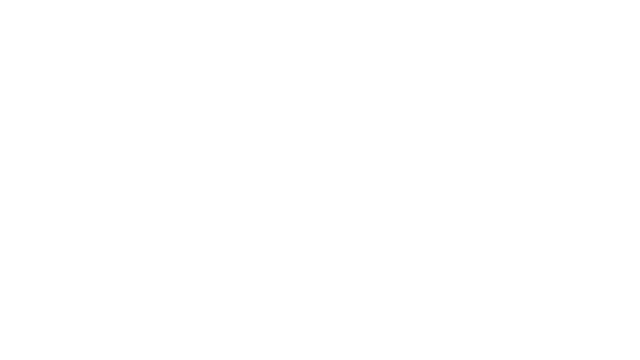 anyone viewing the shot. A low shot looking up at a subject can give that subject a sense of dominance and of power. Cropping in close to someone's face can make a shot feel more intimate and more claustrophobic. Having a subject surrounded by a lot of space can make them feel 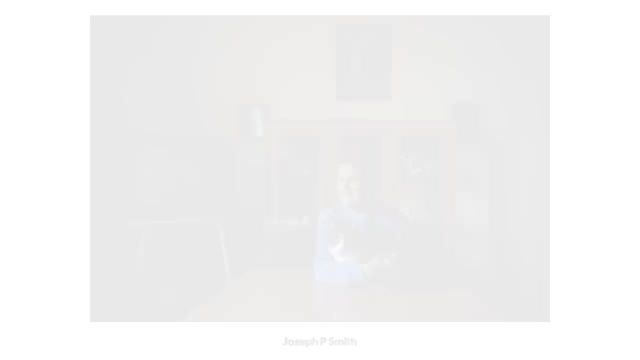 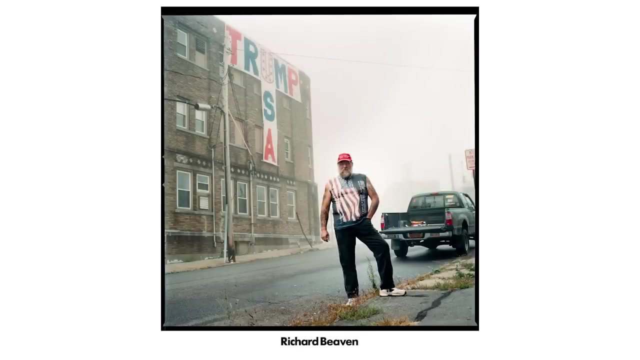 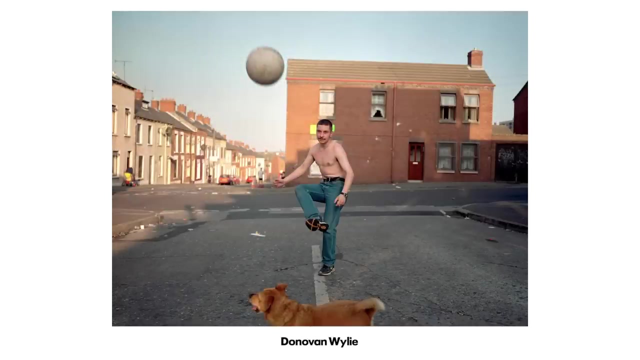 more vulnerable and more defined by their environment. Sometimes, moving further away or using a wider lens can add some wider story to your shot. Decide whether context is important. Are you making social or political commentary about the subject? You might want to consider showing something in relation to its surroundings. 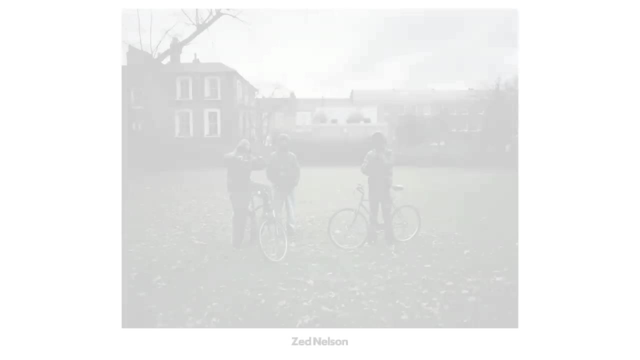 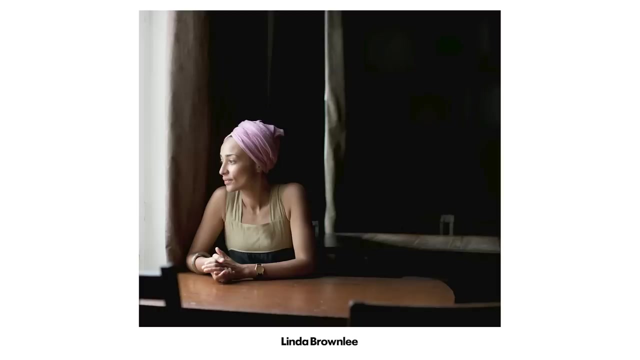 But when making your subject smaller in the frame, be careful, as your subject should probably still be the focal point of your image. You can achieve this by using light contrast, colour leading lines or any of the other tried and tested techniques to draw the viewer's eye to your. 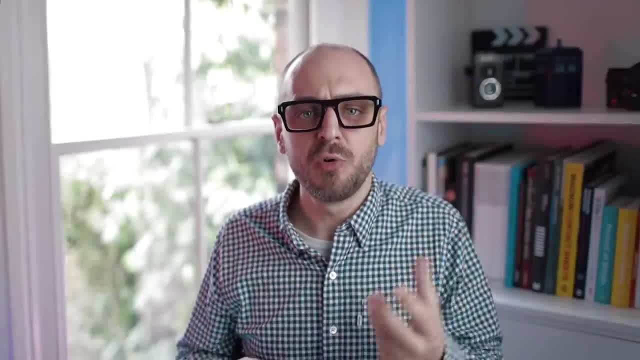 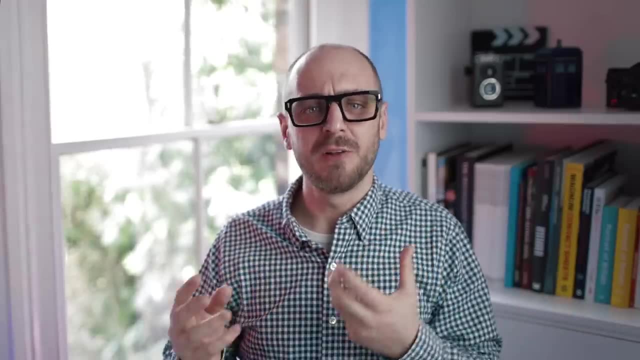 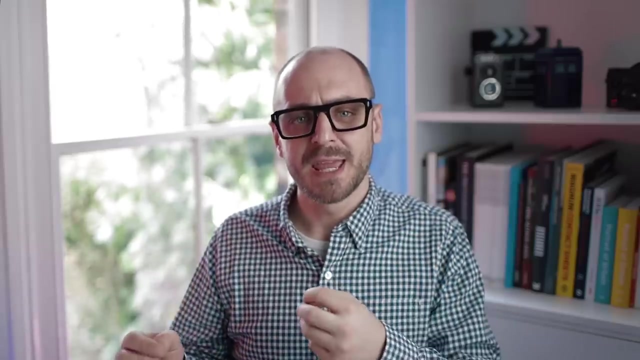 subject. Maybe employing those mathematical compositional rules will make your image feel perfectly balanced. But what if you don't want it to feel perfectly balanced? What if you want your image to feel uneasy because of the subject matter of the photograph? Always consider what you want your image to say before you decide how to say it. 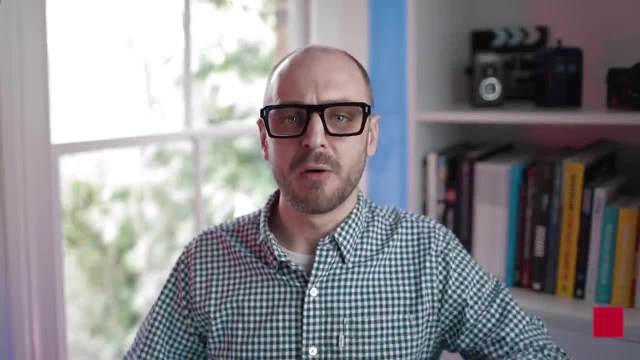 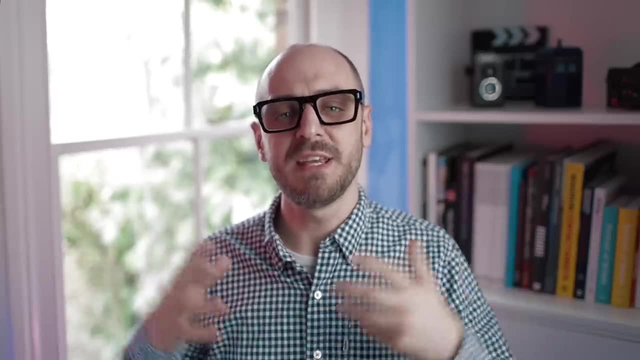 Six keep it simple. In slight contrast to my previous point about showing wider context, a really common compositional mistake I see is people including too much irrelevant detail in the frame. Everything in the frame should be relevant. It should be part of the story. 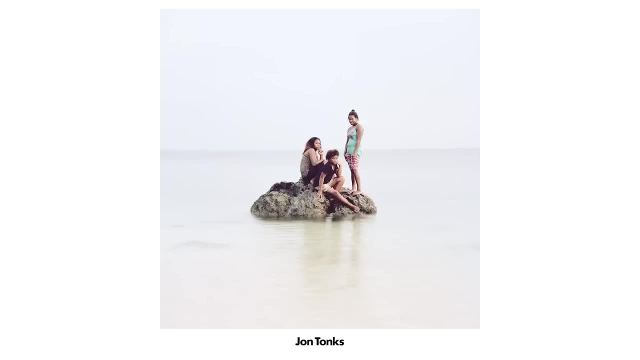 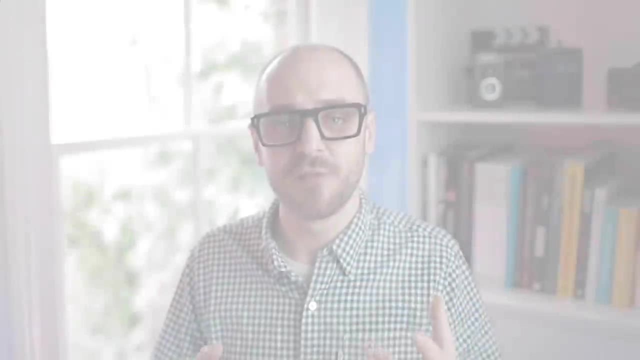 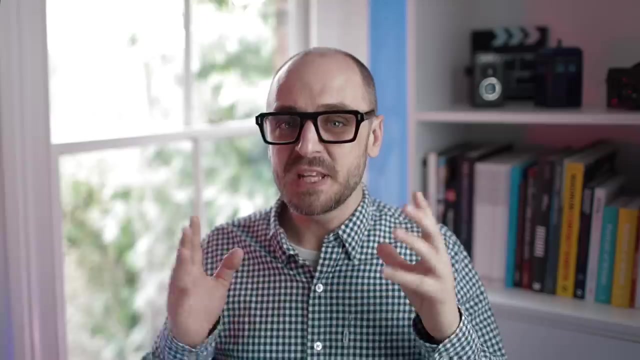 If it's not get rid of it. Seven try to make your subject feel the frame. The act of composing a shot is in itself a form of editing. Your audience won't know what they can't see. Throwing stuff away can be difficult. 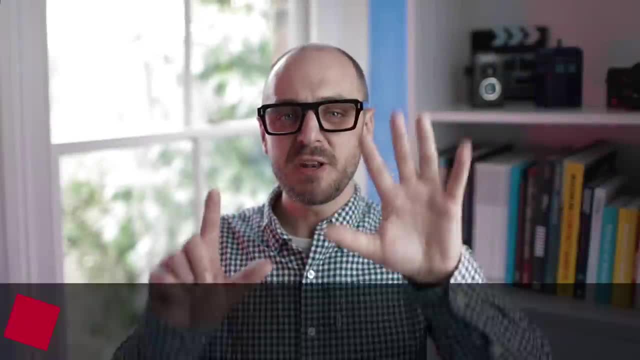 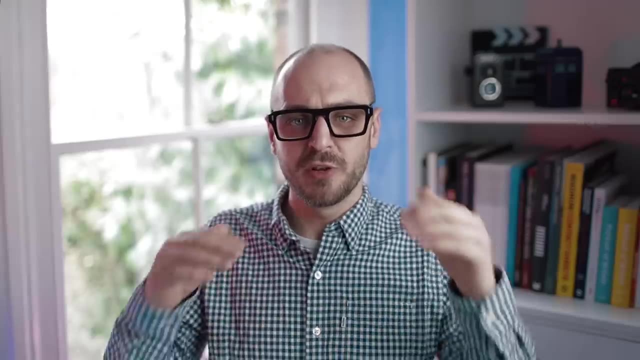 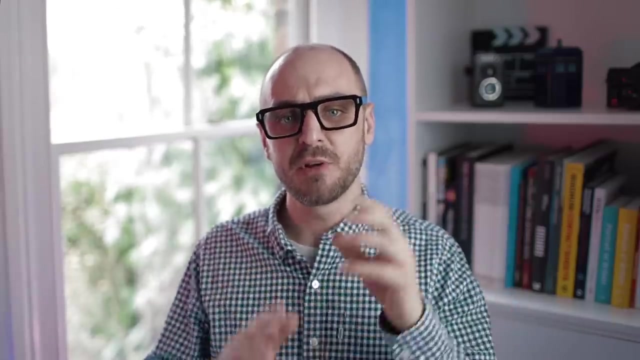 but it can also be very liberating. Seven: watch the edges. Pay particular attention to the borders of your frame. Try not to cut off people's elbows or the top of someone's hair, or the top of trees or buildings or whatever it is you're photographing. Distracting elements at the edge of the frame can draw the 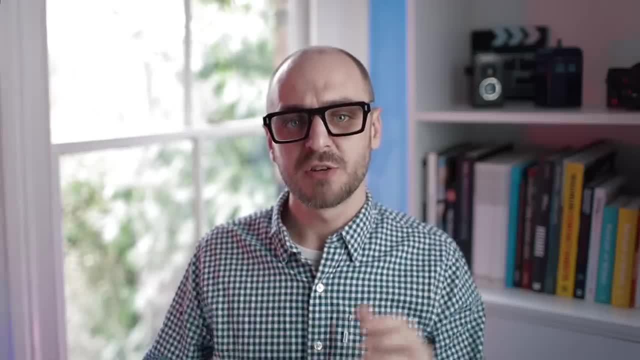 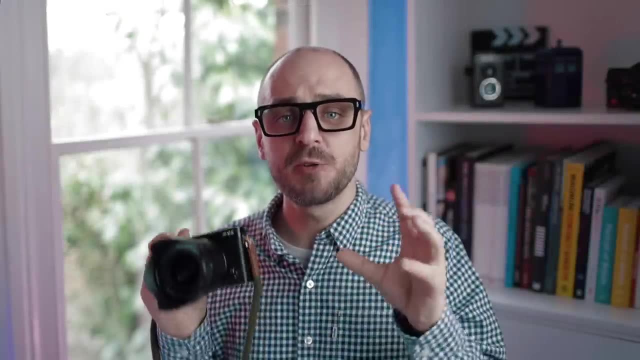 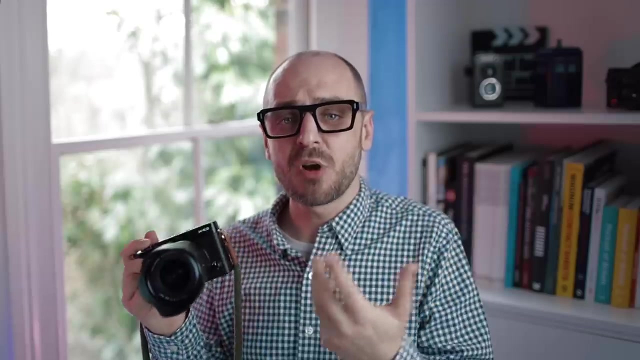 viewer's eye away from your point of focus, So try and keep them clean. Eight work in post. Don't be afraid to also work in post-production to get that perfect composition. You can crop, you can re-level your image. Of course it's better to do it in camera. 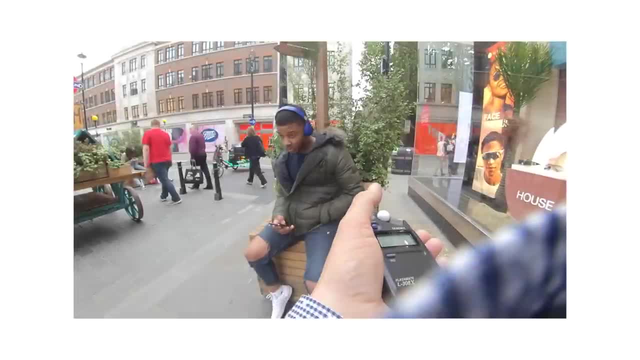 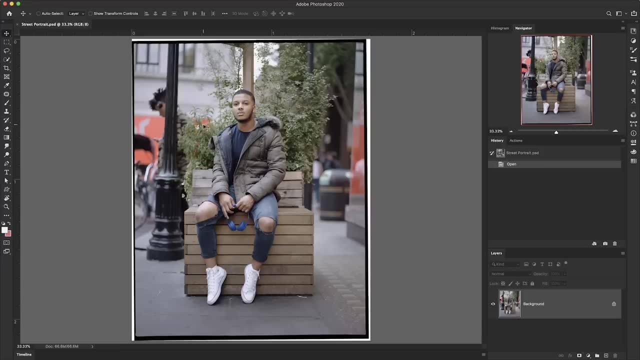 but you have quite a lot of options in post-production. Taking time to compose your shot is important, but so is not missing the moment. The more you crop in post, the better you will become at judging composition in camera. Try testing your shot by flipping the image into a mirrored view. Try inverting the colours. Try. 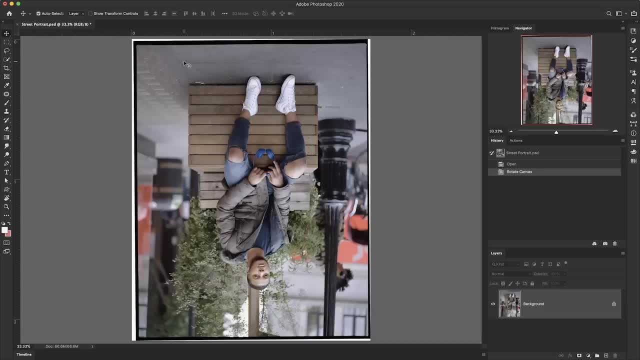 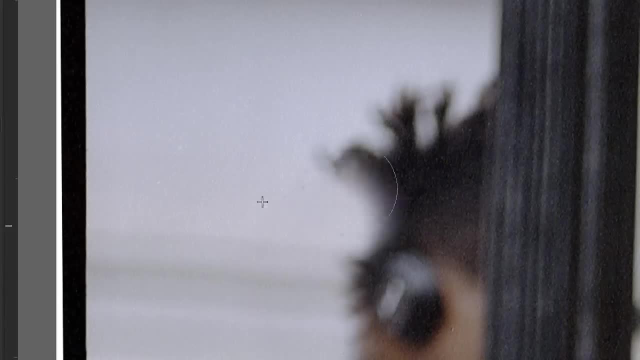 turning it upside down, Does it still feel balanced? And while cropping in post is great, also, don't be afraid to photoshop out elements that are making your shot unbalanced or creating tension by being too near the edge If there's something brightly coloured in the background, 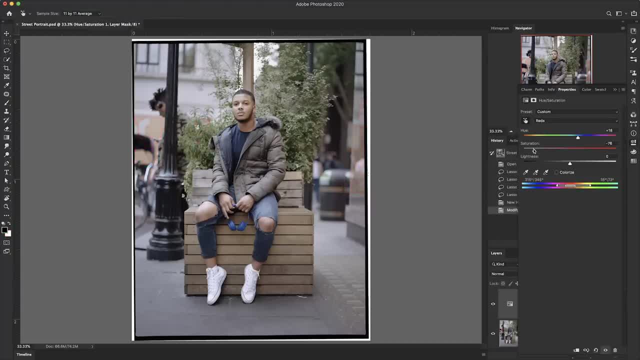 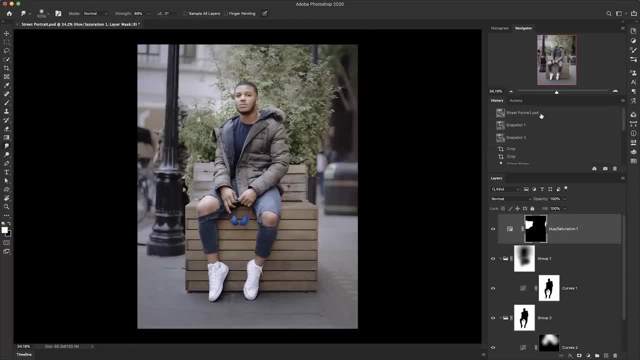 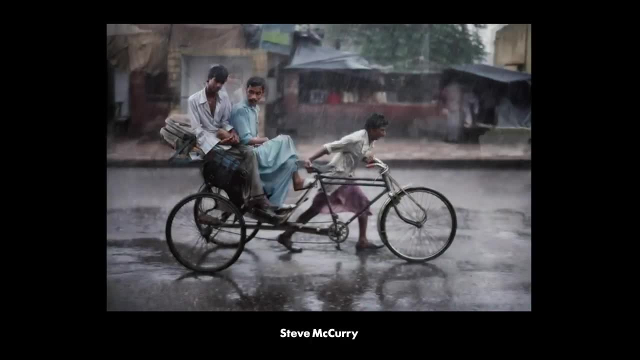 Steve McCurry does this all the time. You could argue it's cheating and by all means follow your own set of ethics and values, but be aware that you are making things harder for yourself. It's up to you, But the key thing here is practice. There are so many compositional rules that you can't. 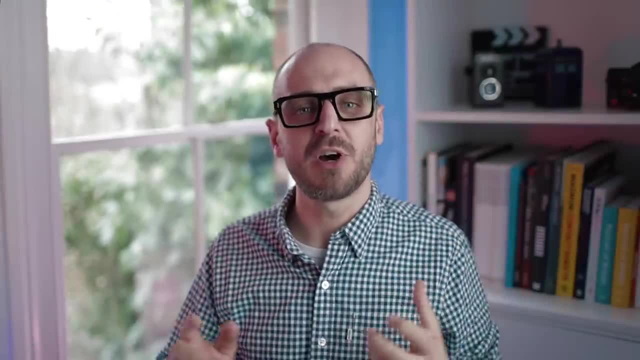 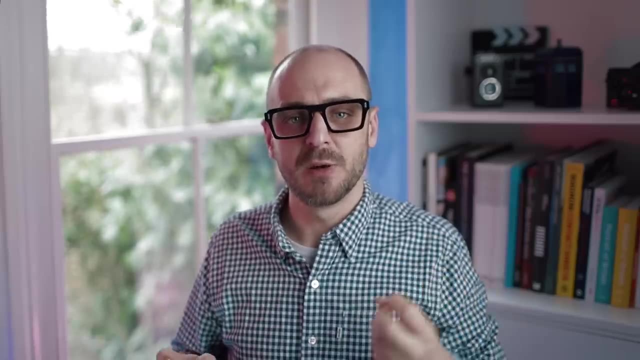 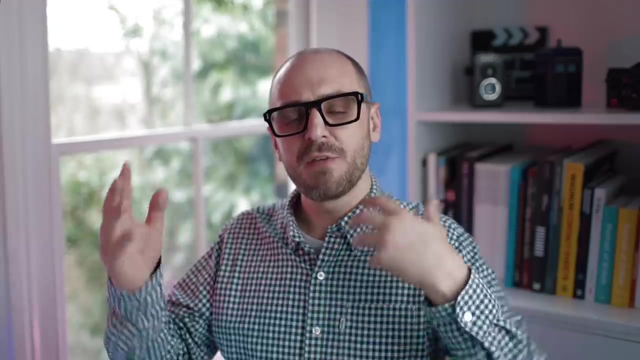 possibly consciously think about every single one every time you take any photograph. But do take time to learn them. Do take time to practice them. Learn one at a time, Go out and try practicing that particular one and eventually you'll kind of absorb them all and they will become. 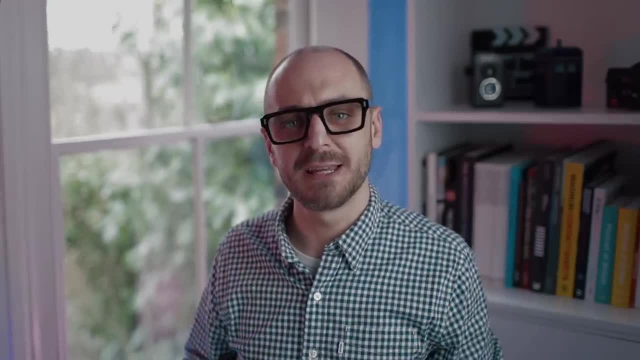 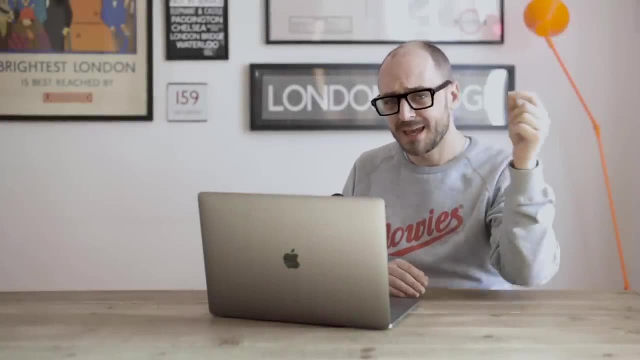 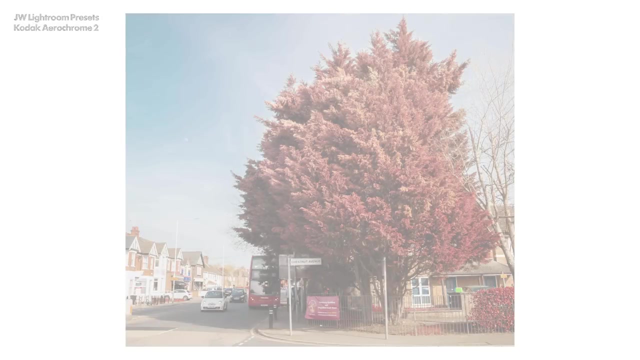 kind of a natural part of your intuitive visual understanding. So a massive thank you to everyone who supports me on Patreon- You guys are the absolute best- and also a big thank you to anyone who's bought my Lightroom preset packs, because those both help fund this channel and keep me. 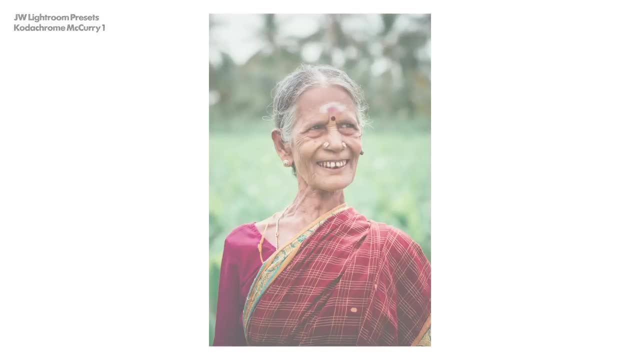 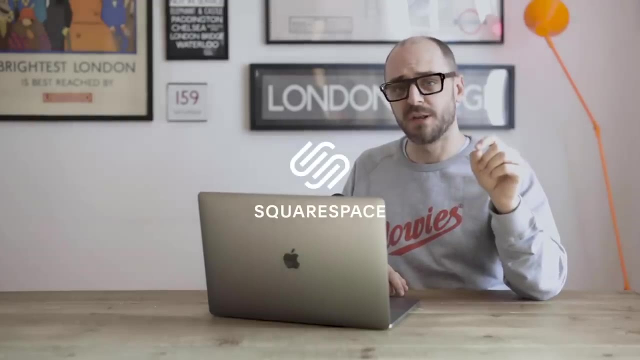 making videos. If you want to have a look at my presets, then I'll put a link down below this video which will take you to my website. My website was built on Squarespace, which is the sponsor of this video. Squarespace is an all-in-one web hosting platform. I've been using Squarespace for many. 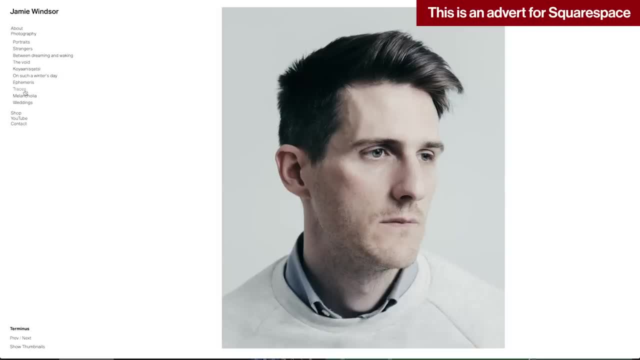 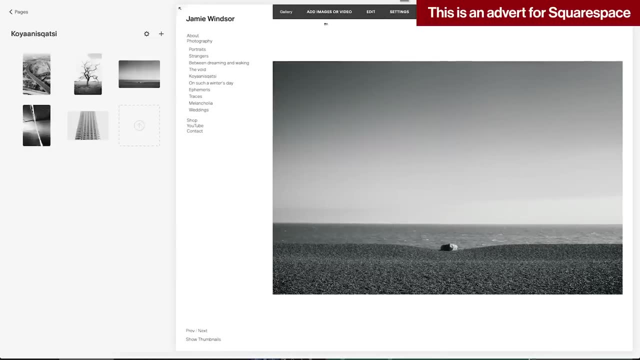 years, and so do many professional photographers, designers, filmmakers, etc. There's no software or patches to install. It's all done through your browser, so you can easily update your site from wherever you are. as long as you have an internet connection, You can easily keep up to date with. 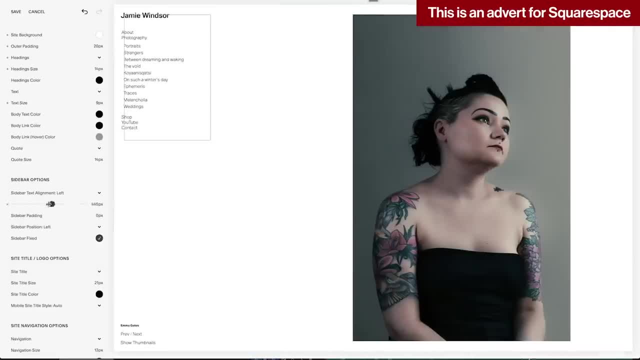 your analytics or you can even manage sales through your site, as they offer a range of e-commerce tools. The website tells you how to use Squarespace and how to use it. You can also use Squarespace to manage sales through your site, as they offer a range of e-commerce tools. The website tells: 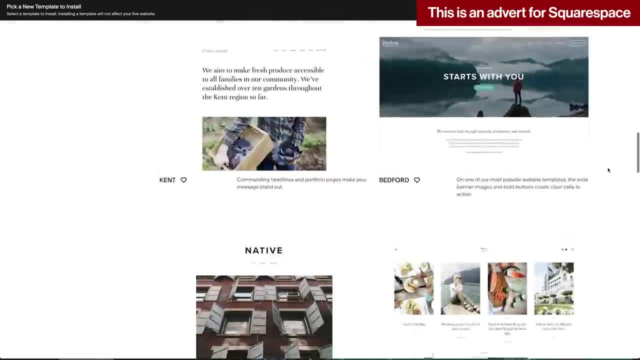 you how to manage sales through your site, as they offer a range of e-commerce tools. The website tells templates are really nicely designed and are customizable, but you can also paste in your own bespoke css code if you want to add some extra functionality, like I've done here with this before. 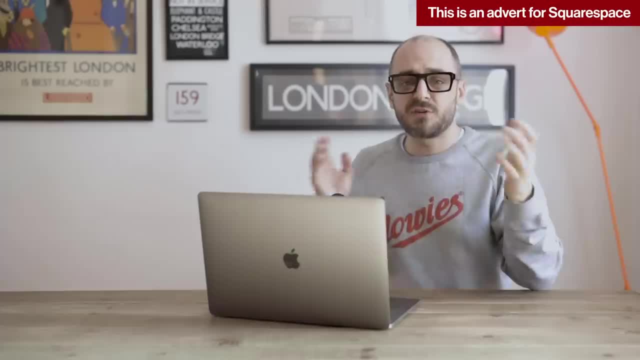 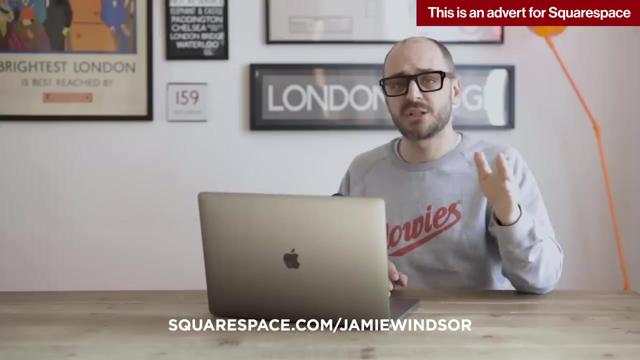 and after slider to show my Lightroom presets. So if you want to give Squarespace a go, they offer a completely free trial. so you just go to squarespacecom and you can start building your site and see how easy it is. and if you like it, you can go to squarespacecom forward slash Jamie Windsor.